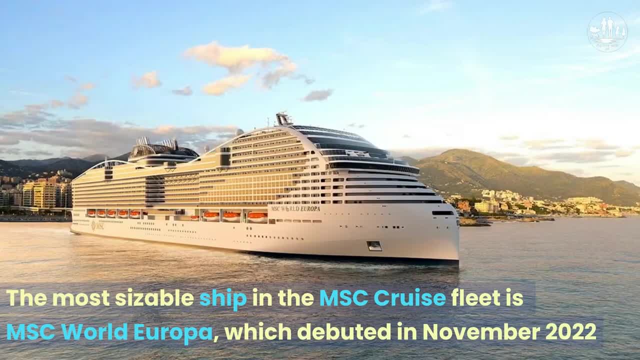 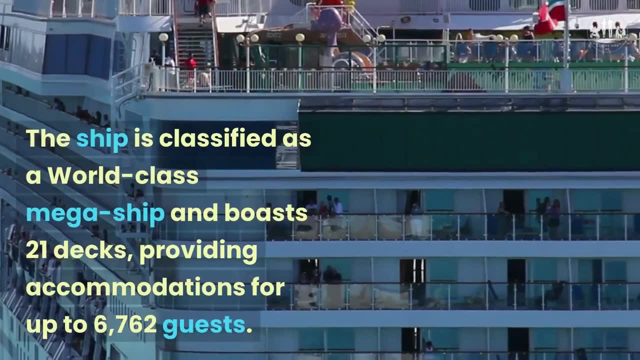 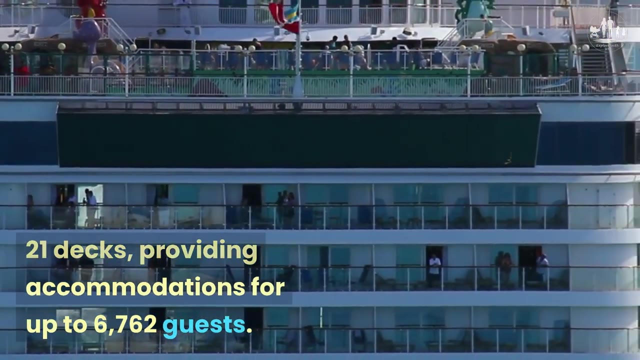 The most sizable ship in the MSC cruise fleet is MSC World Europa, which debuted in November 2022.. The ship is classified as a world-class cruise ship. It is the world's largest mega ship and boasts 21 decks providing accommodations for up to 6,762 guests. 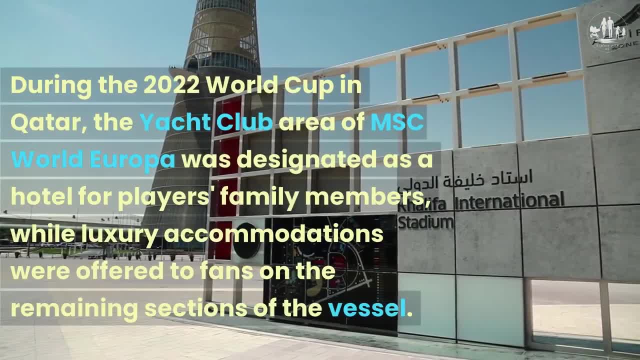 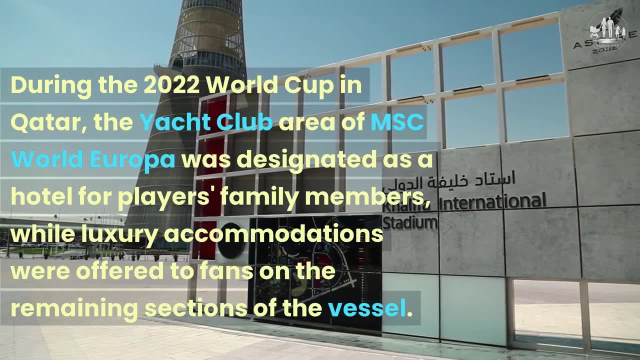 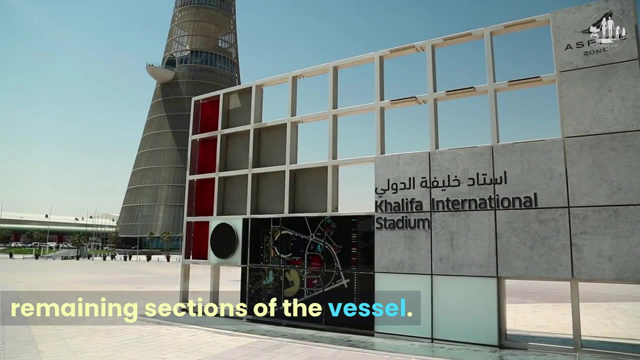 During the 2022 World Cup in Qatar, the yacht club area of MSC World Europa was designated as a hotel for players' family members, while luxury accommodations were offered to fans on the remaining sections of the vessel. What is MSC World Europa? Although MSC World Europa is the sixth-largest cruise ship globally, it is the world's largest cruise ship in the world. 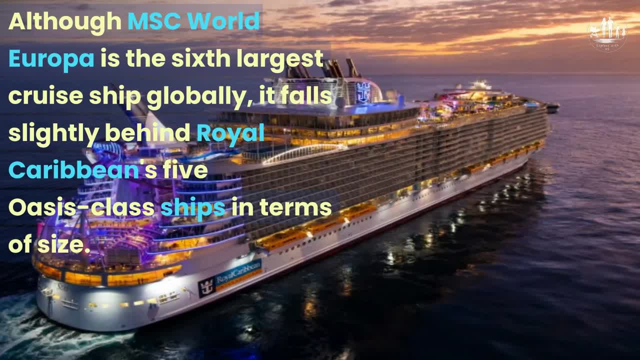 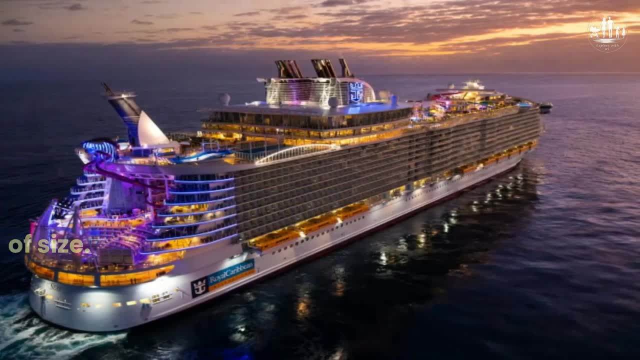 What is MSC World Europa? MSC World Europa is the world's largest cruise ship in the world. Sadly, it falls slightly behind Royal Caribbean's five Oasis-class ships in terms of size. However, MSC World Europa is larger than its peers' ship 9275.. 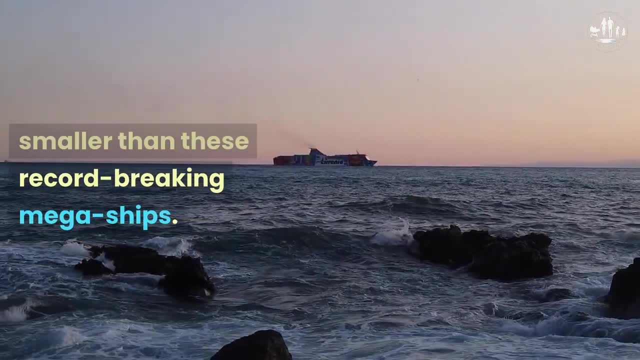 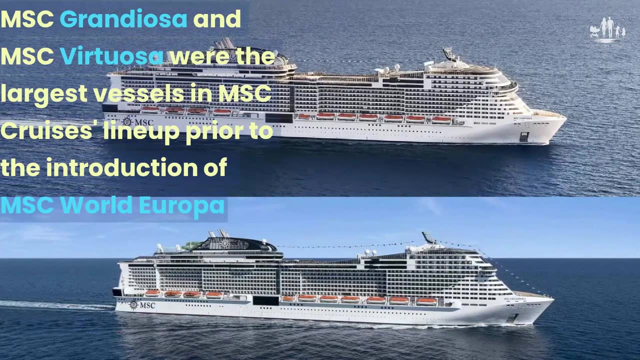 Despite this, MSC World Europa is only approximately 5 per cent smaller than these record-breaking mega ships. MSC Grandiosa and MSC Virtuosa were the largest vessels in MSC Cruiser's lineup prior to the introduction of MSC World Europa. MSC Grandiosa and MSC Virtuosa were the largest vessels in MSC Cruiser's lineup prior to the introduction of MSC World Europa. 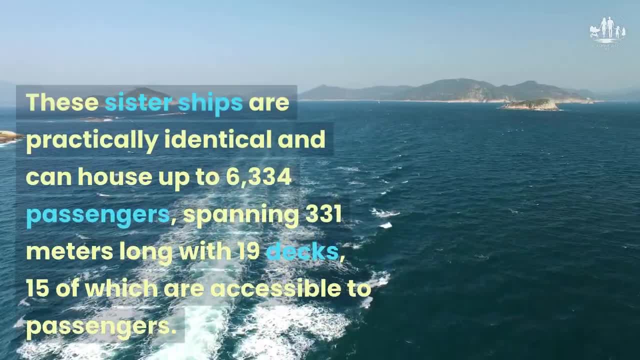 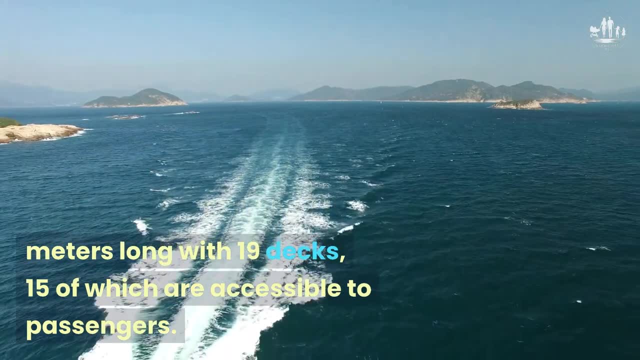 These sister ships are practically identical and can house up to 6,636 passengers. Although MSC World Europa is the world's largest cruise ship, it quien-expelled and colour-coded in Kingdom Rebellion. up to 6,334 passengers, spanning 331 meters long, with 19 decks, 15 of which are accessible. 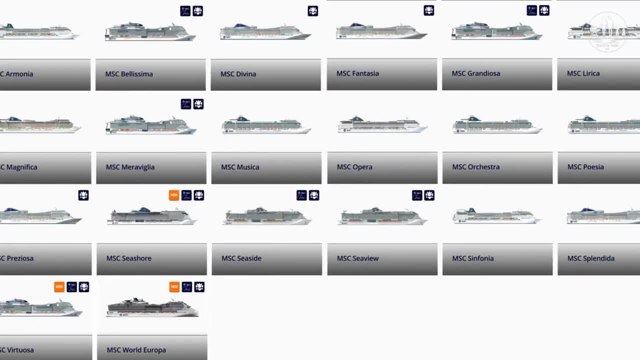 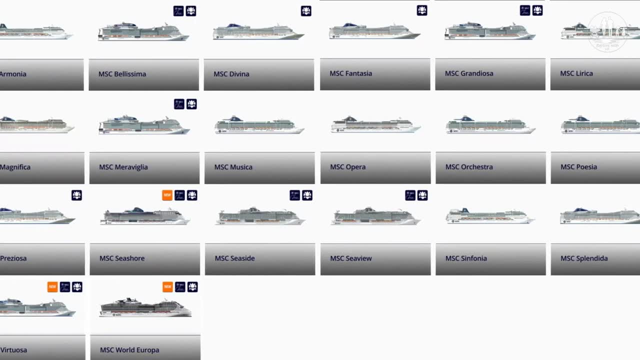 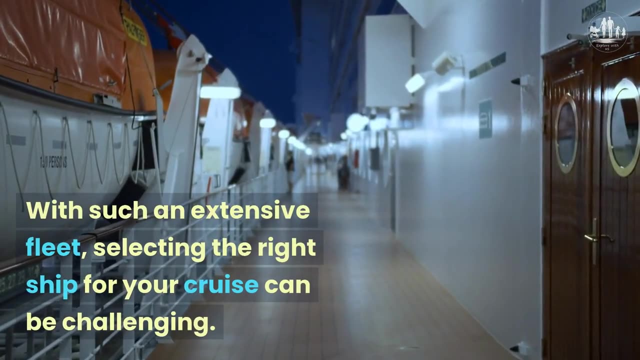 to passengers In the year 2023,. MSC Cruises is operating a fleet of 21 ships, and another vessel is expected to launch this year, bringing the total number of ships in the fleet to 22.. With such an extensive fleet, selecting the right ship for your cruise can be challenging. 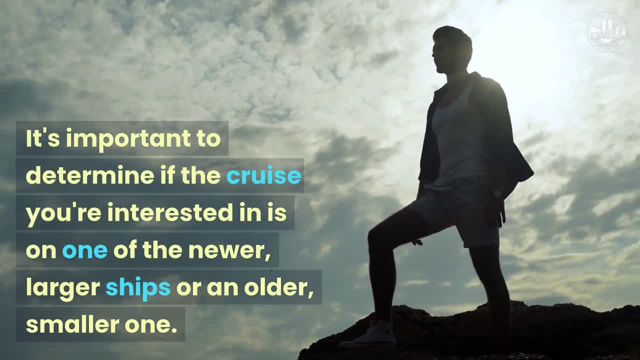 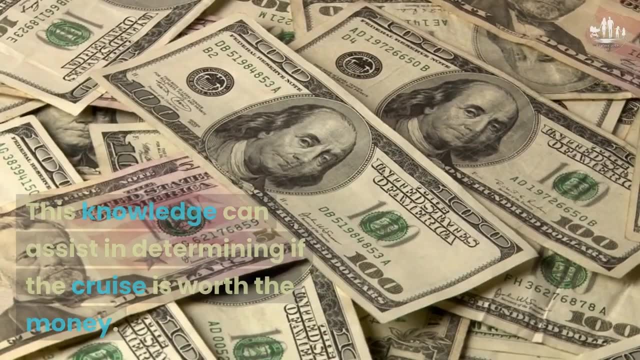 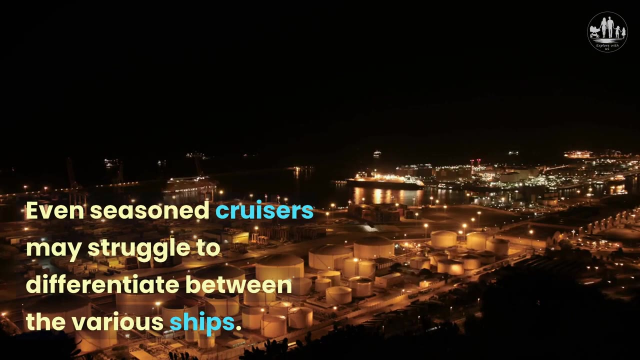 It's important to determine if the cruise you're interested in is on one of the newer, larger ships or an older, smaller one. This knowledge can assist in determining if the cruise is worth the money. Even seasoned cruisers may struggle to differentiate between the various ships. 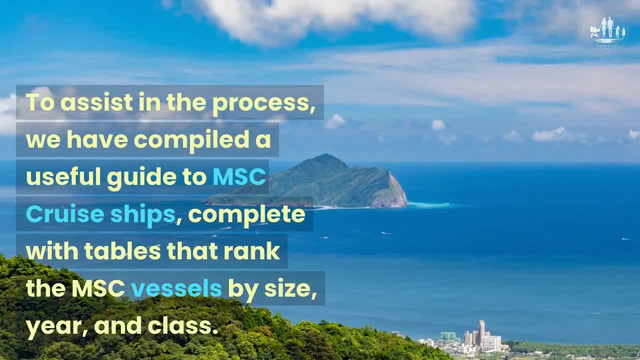 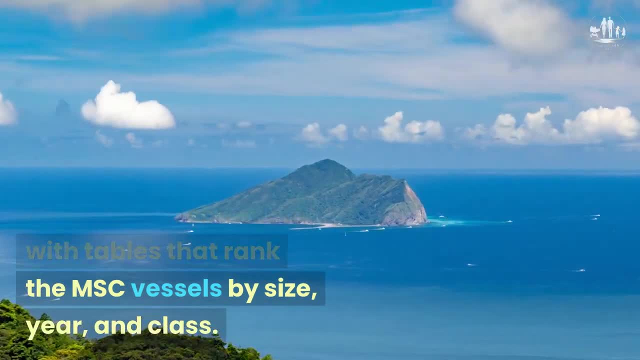 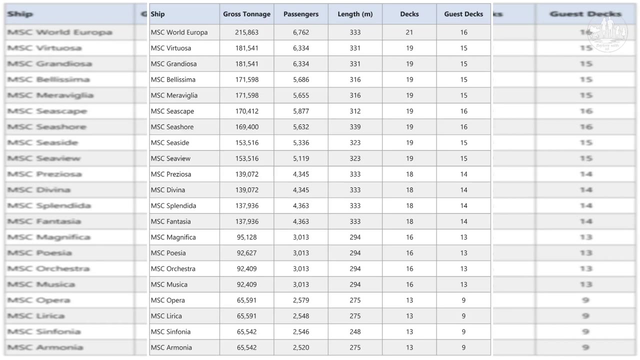 To assist in the process, we have compiled a useful guide to MSC cruise ships, complete with tables that rank the MSC vessels by size, year and class. Displayed is a table of MSC Cruises ships arranged according to their size, from the 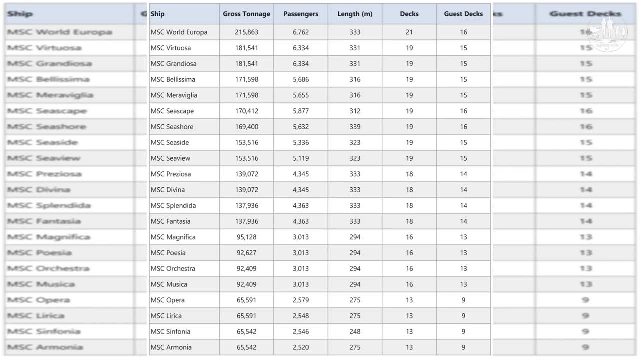 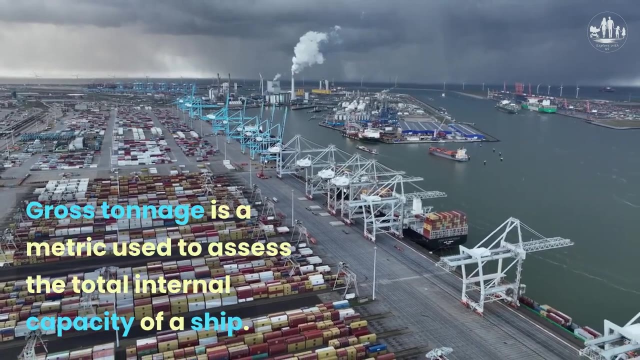 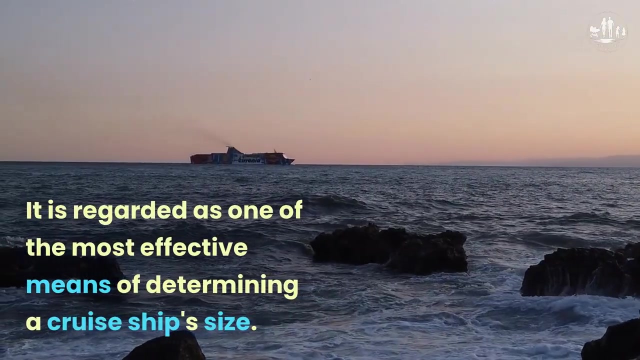 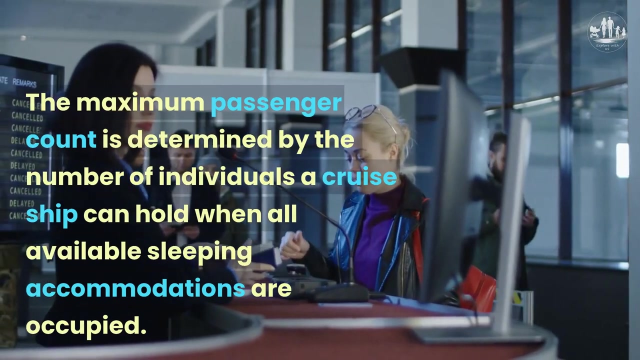 biggest to the smallest vessel. 1. Gross tonnage is a metric used to assess the total internal capacity of a ship. It is regarded as one of the most effective means of determining a cruise ship's size. 2. The maximum passenger count is determined by the number of individuals a cruise ship. 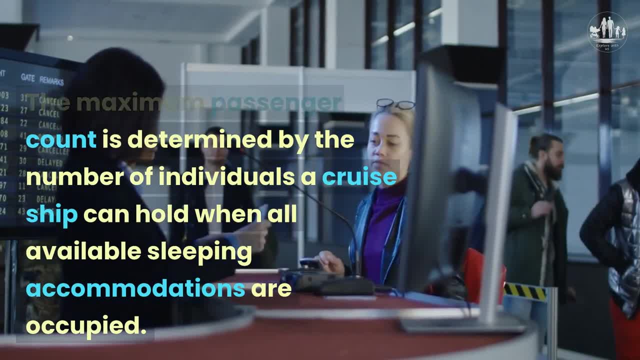 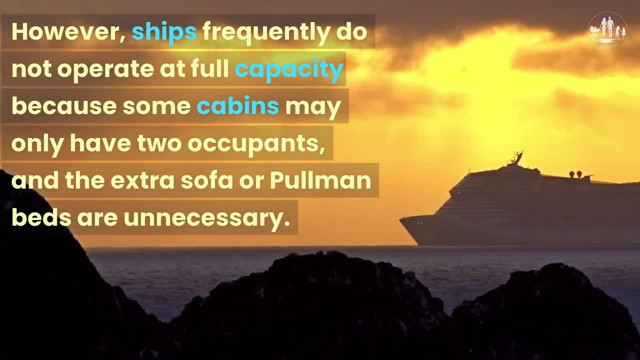 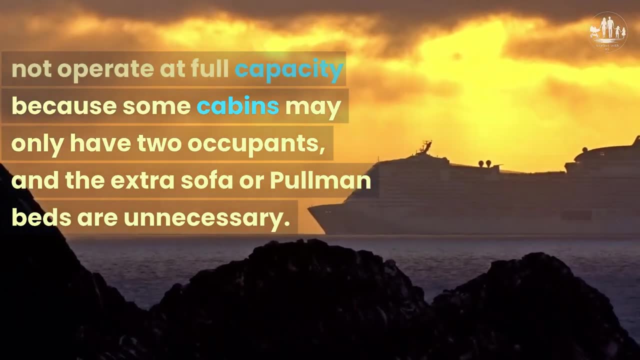 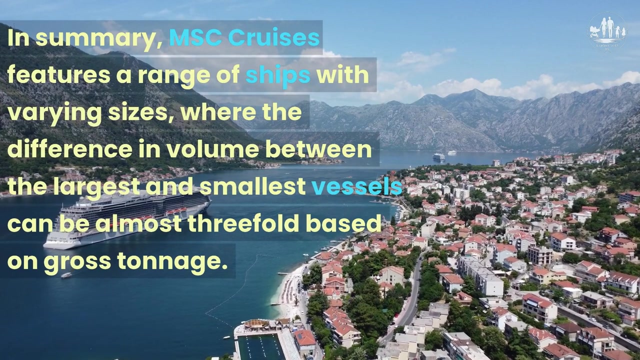 can hold when all available sleeping accommodations are occupied. 3. Ships frequently do not operate at full capacity because some cabins may only have two occupants and the extra sofa or Pullman beds are unnecessary. In summary, MSC Cruises features a range of ships with varying sizes. where the difference 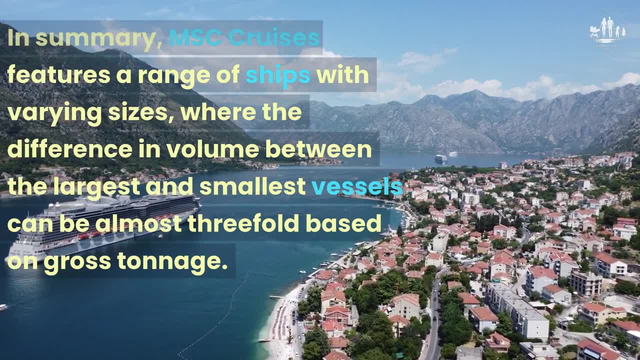 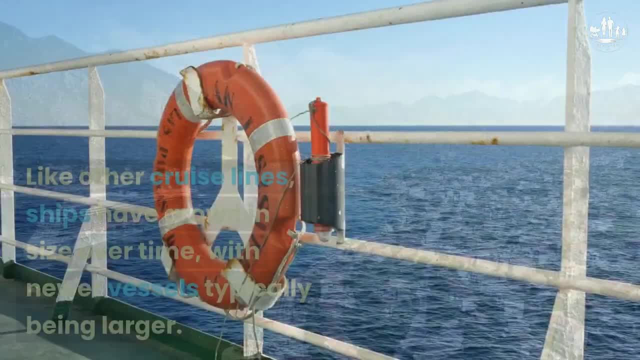 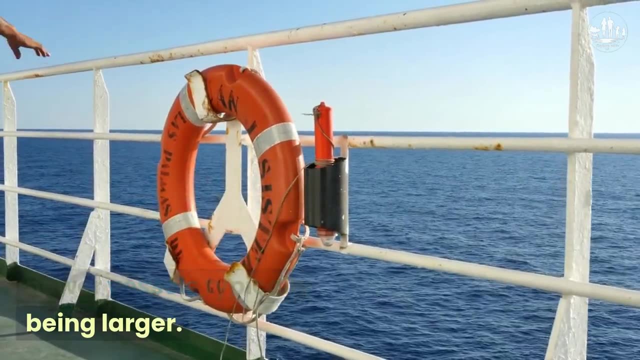 in volume between the largest and smallest vessels can be almost threefold based on gross tonnage. Like other cruise lines, ships have grown in size over time, with newer vessels typically being larger. For those who prefer smaller, more personalized ships, the MSC Group has recently introduced 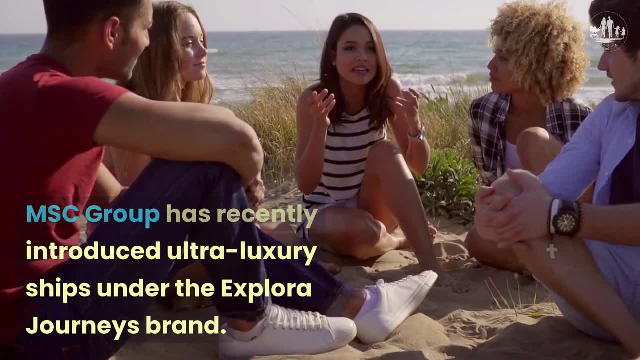 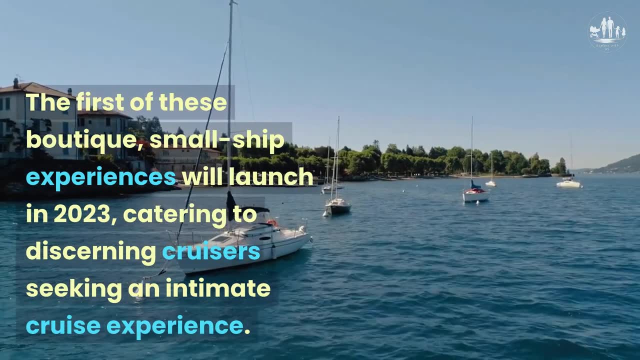 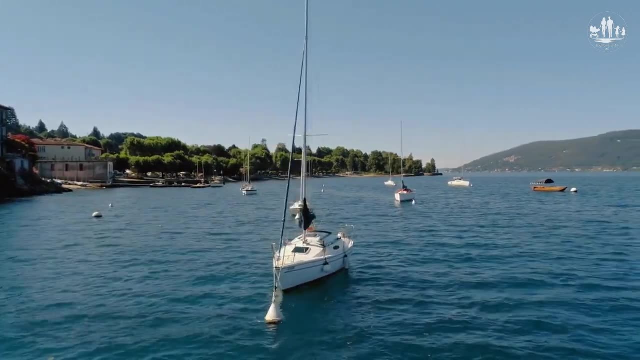 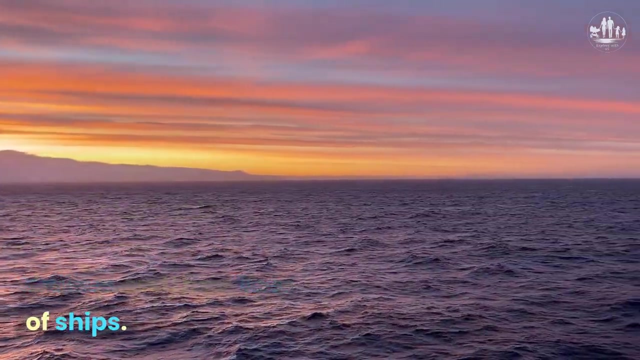 ultra-luxury ships under the Explorer Journeys brand. The first of these boutique small-ship experiences will launch in 2023, catering to discerning cruisers seeking an intimate cruise experience. Thanks for watching. Thank you for watching our video about MSC Cruises and their fleet of ships. 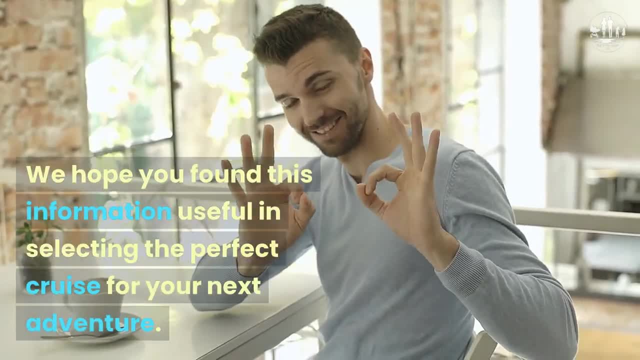 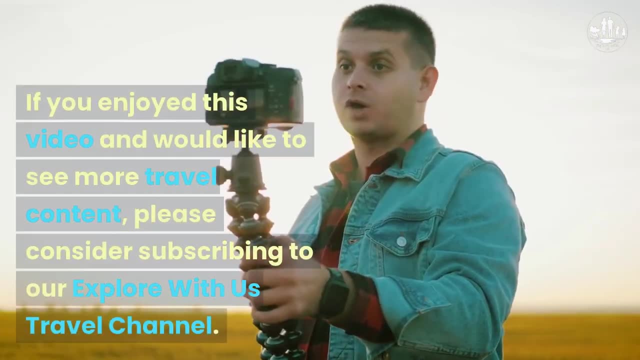 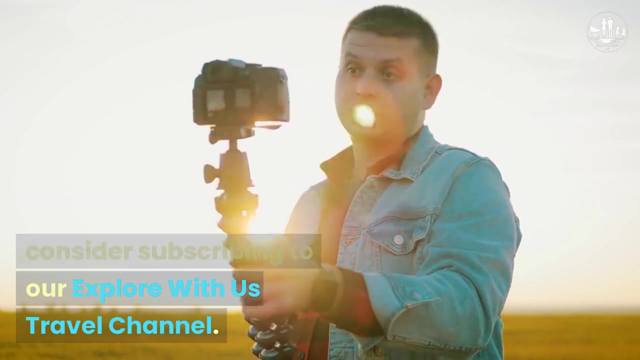 We hope you found this information useful in selecting the perfect cruise for your next adventure. If you enjoyed this video and would like to see more travel content, please consider subscribing to our Explore With Us Travel Channel. Our channel is dedicated to helping you get the most out of your cruise experience.